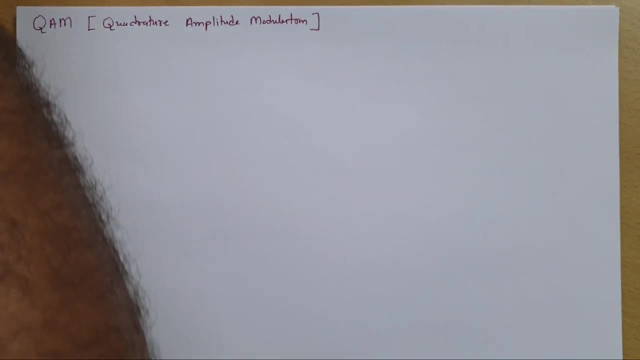 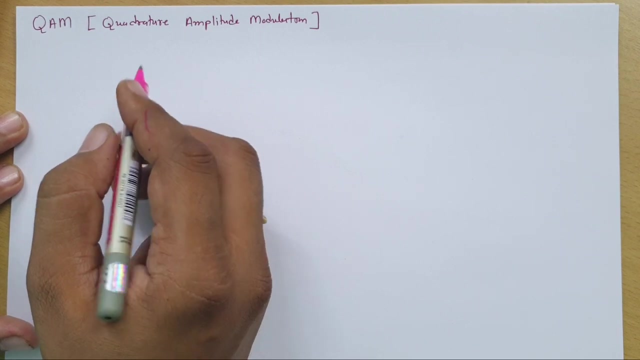 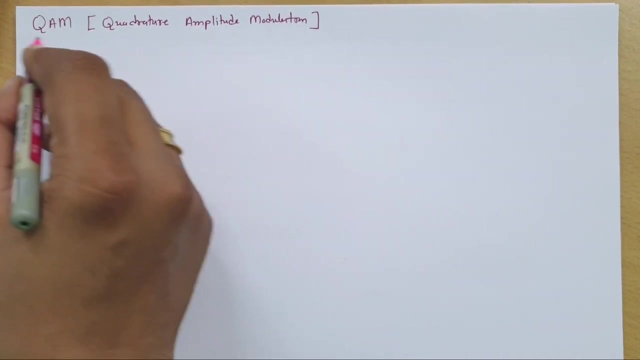 with QAM. so see, when we talk about quadrature amplitude modulation, its name is quadrature amplitude modulation because of here we have two carrier signal which are there in quadrature phase, right. so see, as per the name, carrier signal- let us say we have a carrier signal. 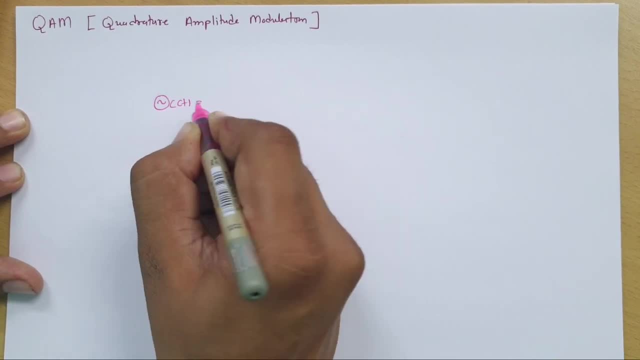 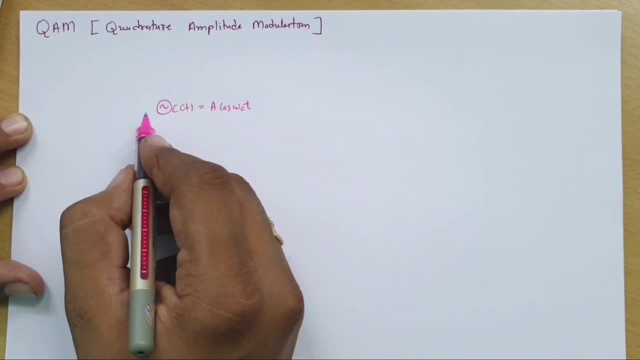 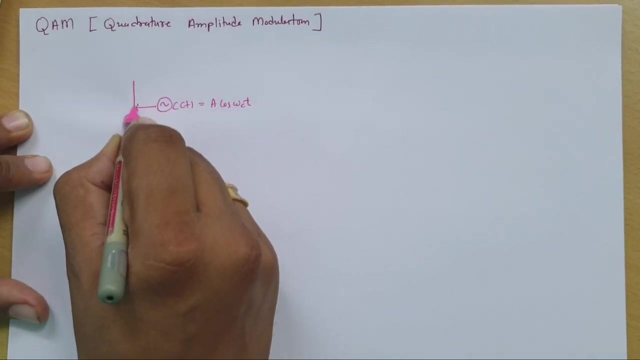 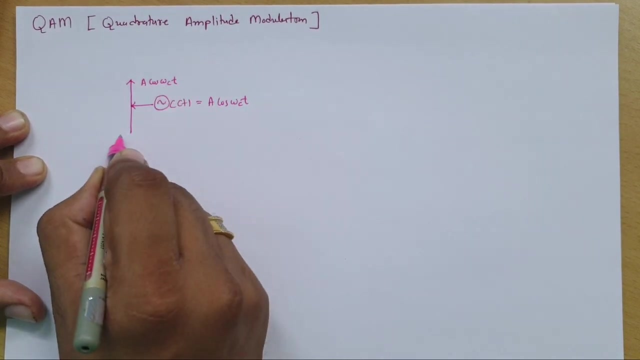 C of T, right, and that is A cos omega C T. so that is what we are translating into quadrature phase. now see how to translate that in quadrature phase. so that we can translate into quadrature phase, as per see over here, there will be A cos omega C T and, if I provide, 90 degree phase. 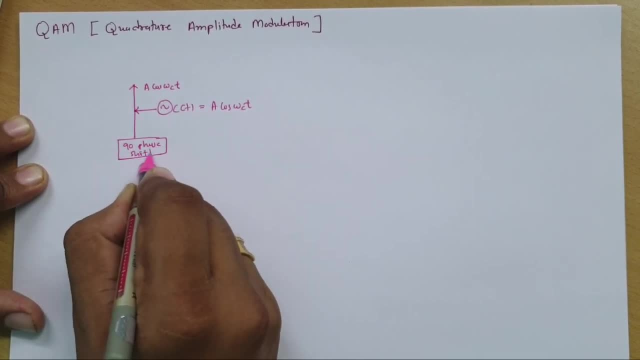 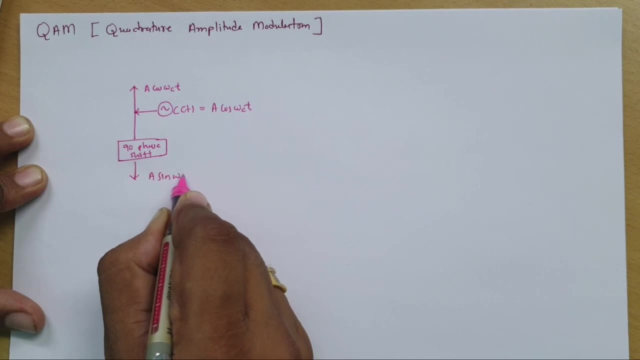 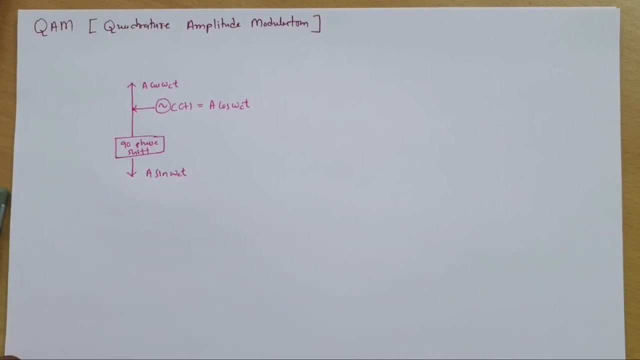 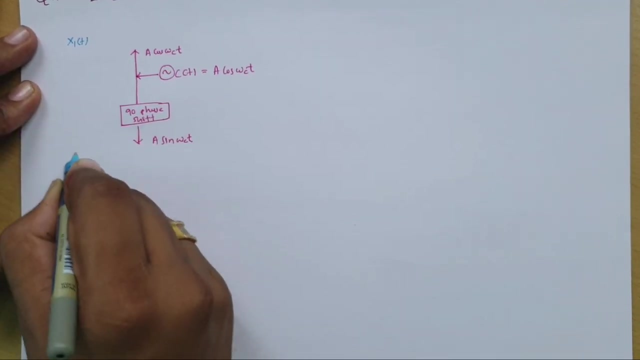 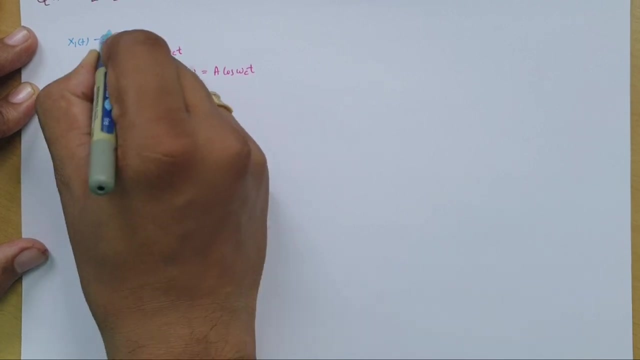 shift. in that case over here my phase will be A sin omega C T, because of 90 degree phase shift is been provided. now see, here in QAM we have two signals over here, let us say x1 T and x2 T, and that signal that we give it over here to this product modulator. 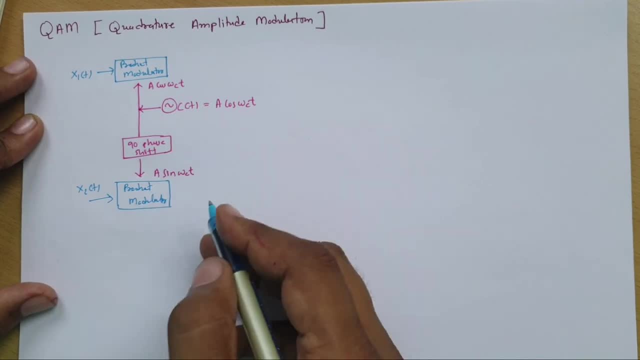 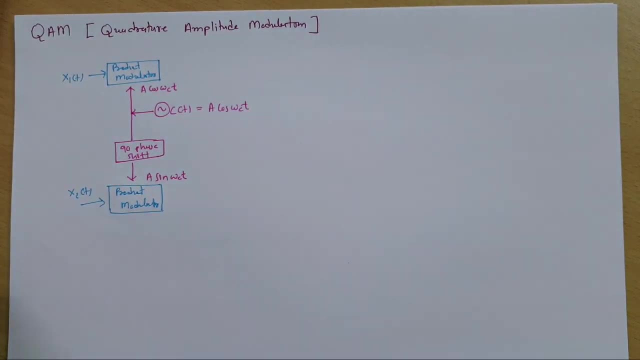 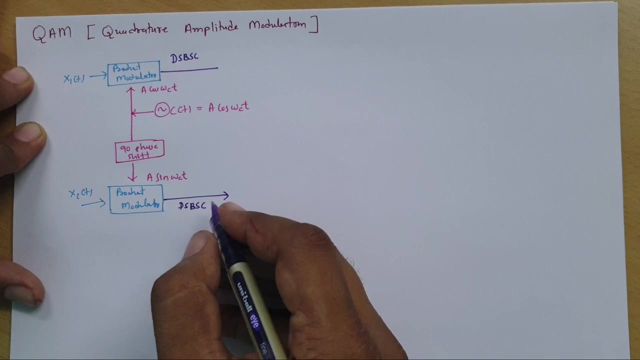 now, as you give this to product modulator, you will be finding at this side. you will be finding at this side. there will be DSBSC output, right, there will be DSBSC output double sideband suppress carrier, and all we will be doing is we will combine this. 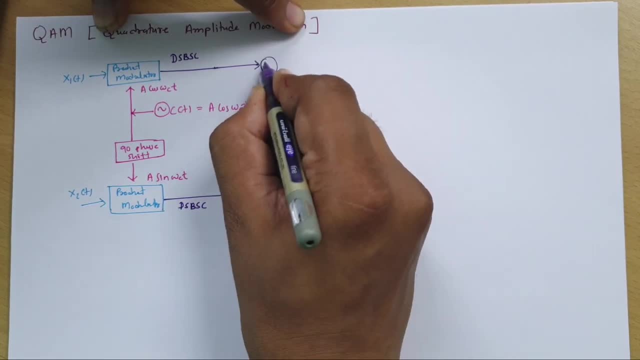 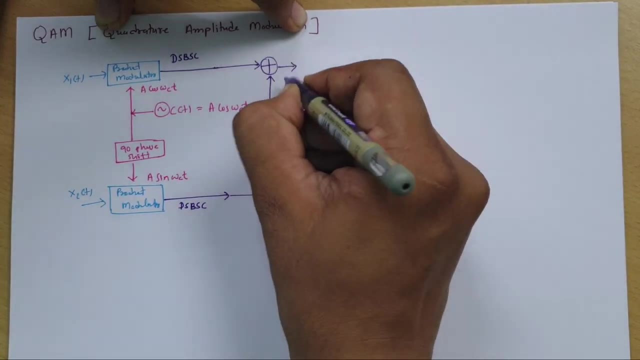 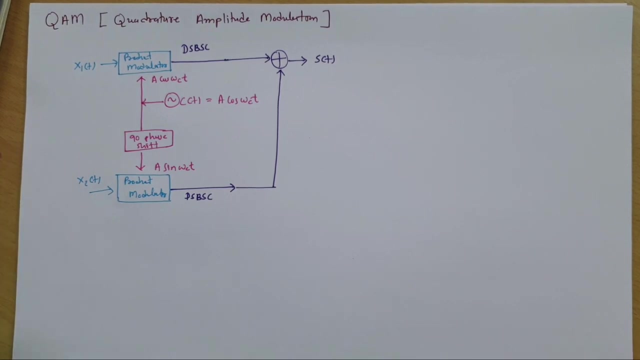 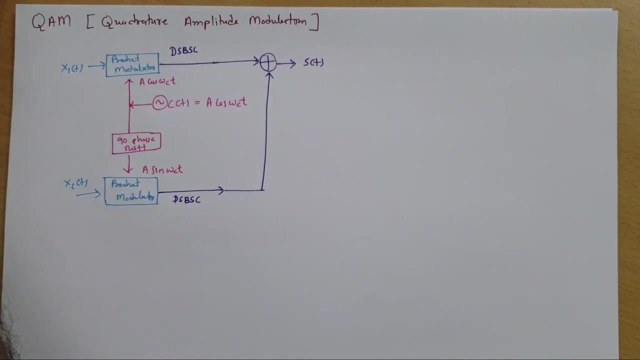 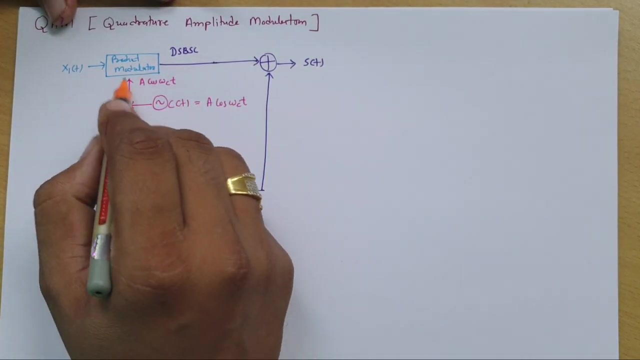 so we will add both of the signals and my resultant signal that will be s of t, my resultant signal that will be s of t, and that is what we are delivered to transmit right now. first thing, that is, we are delivered to understand what is this dsbsc output? that is just a multiplication of inputs as per product modulator, right so? 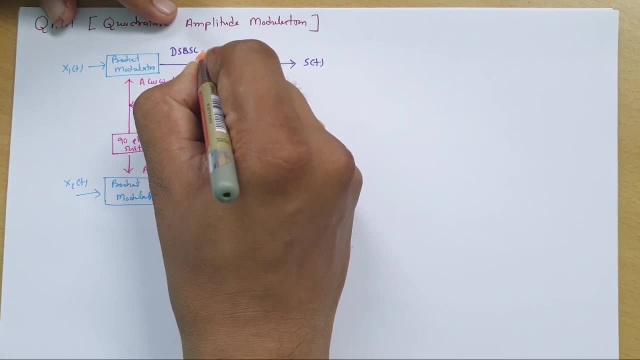 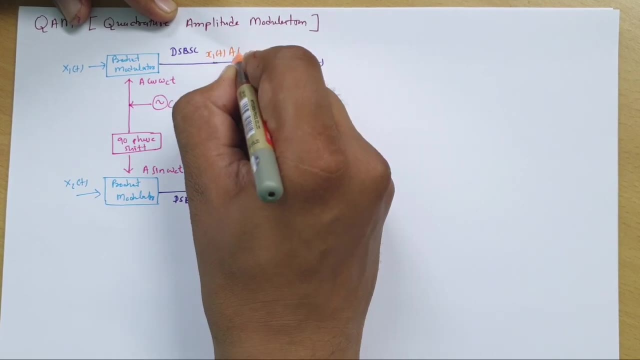 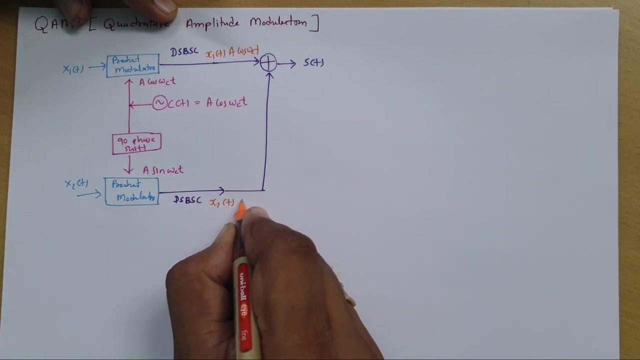 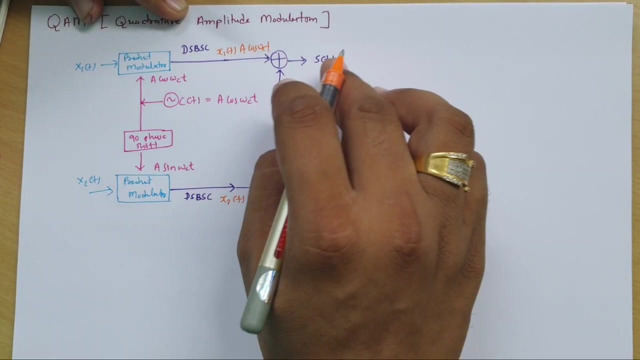 this output. this my first dsbsc output that will be x1 t into a cos omega ct and my second dsbsc output that is x2 t into a sine omega ct and this is just a adder, so we will add it and my s of t that will be addition of this two. so here my output. 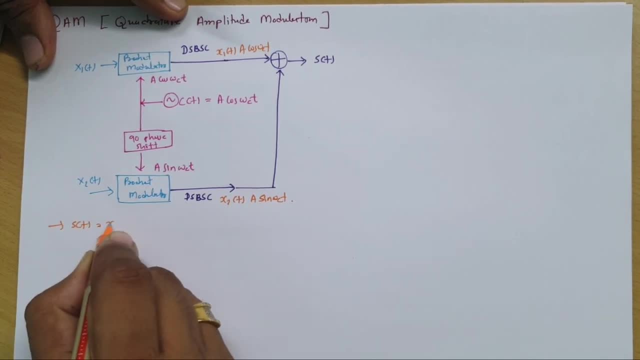 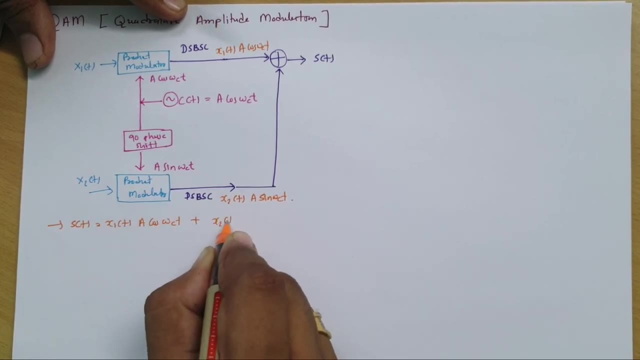 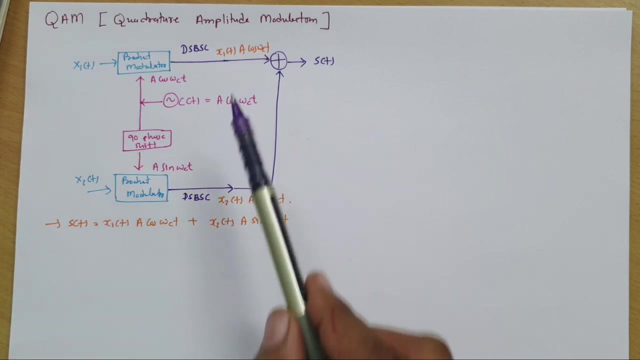 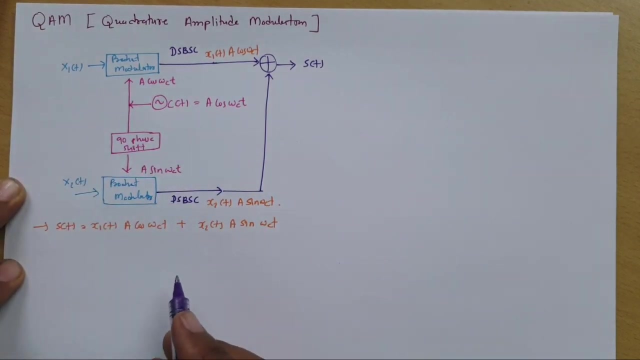 S of t, that is, x1 t into a cos omega ct plus x2 t into a sine omega ct. now see, this is what analog modulation type of diagram right. but when it comes to digital, at that time we will be having digital to analog converter at input side and that will represent analog. 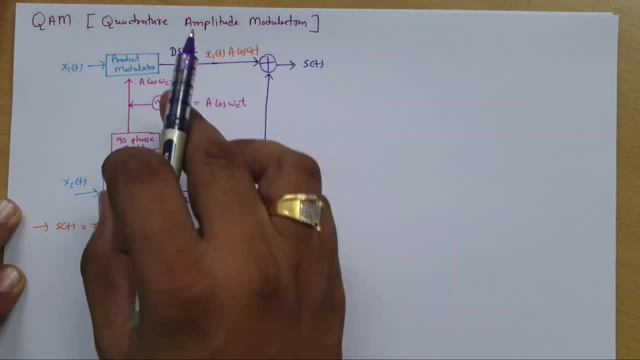 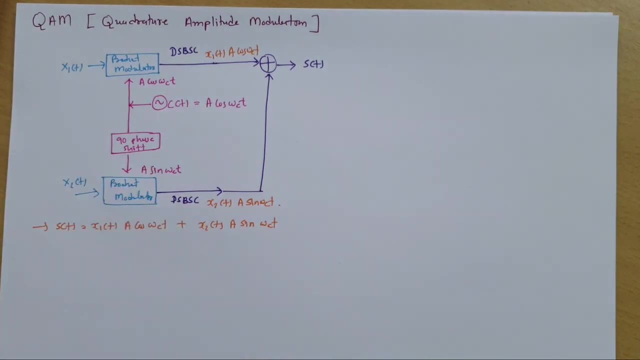 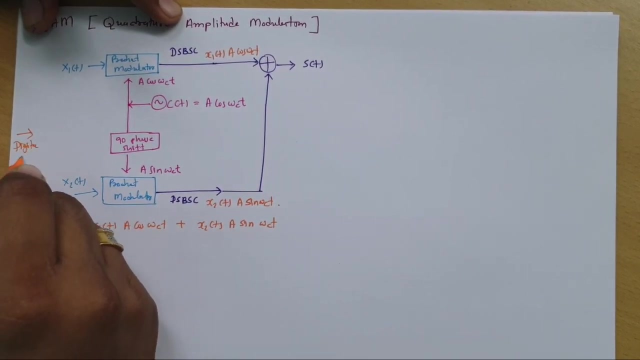 modulator at input side and that will represent amplitude as x1 t and x2 t and that is what we will give it to product modulator. and we will do same thing like see for example here: if i have, here, if i have digital data, then first we will convert this into serial to parallel. let us say serial to parallel. 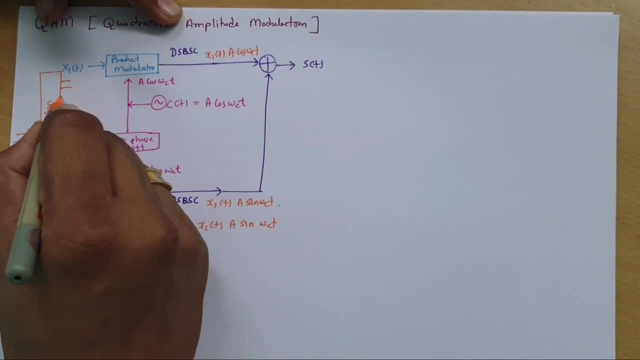 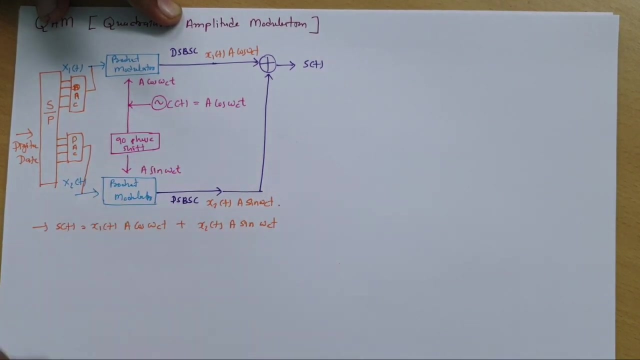 converter is there. After that, once we have serial to parallel conversion, after that there will be digital to analog converter and that is what we will give it as x1 and x2 t. so in digital modulation, this is what the difference which we do, the first. 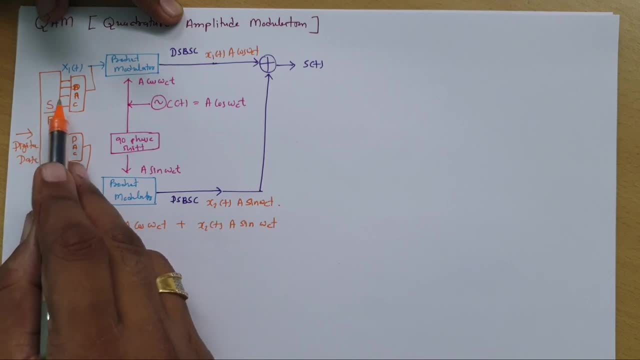 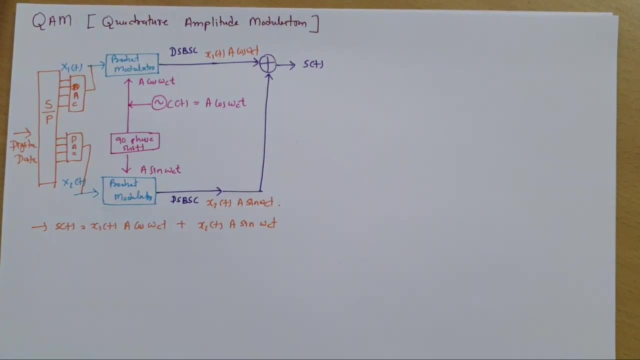 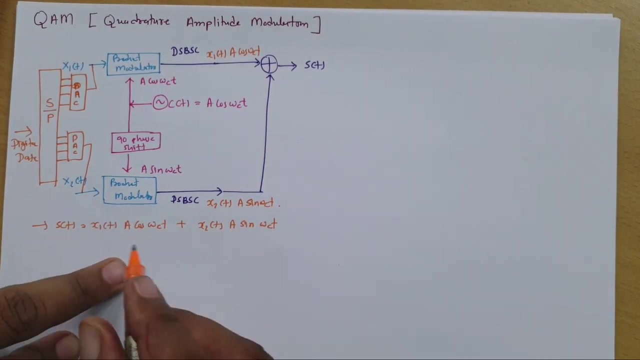 digital data that we convert into parallel, and then digital to analog converter data that we give it over here. so that is what the case, which we do it in digital communication, right? so same thing has been there now. this is what my transmitted data and you can observe. over a same channel, we 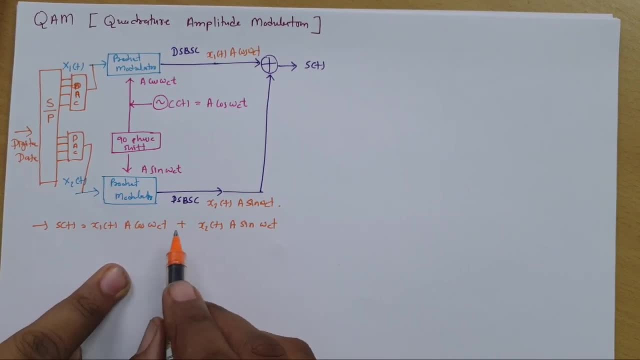 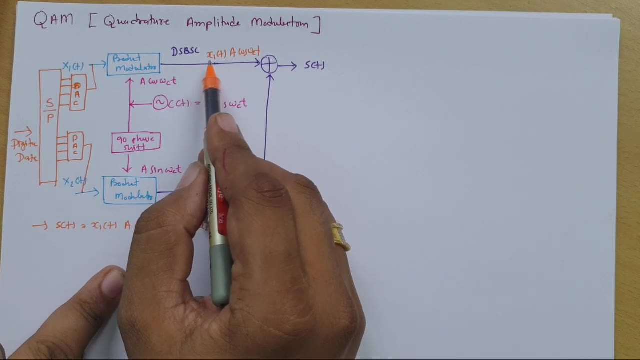 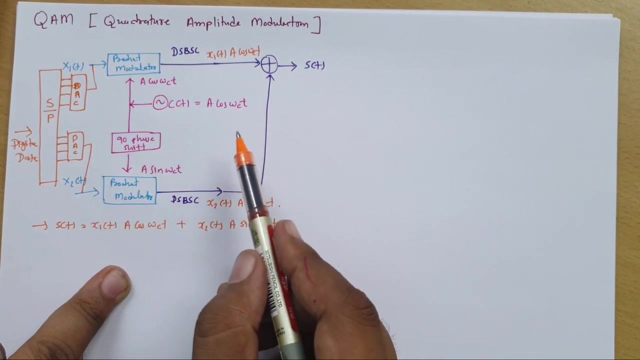 are utilizing bandwidth effectively, right. so here we occupy very less bandwidth. like see in dsbsc, you need bandwidth which is fm, right, but here two dsbsc signal that we are transmitting over a same channel. so here we optimize utilization of bandwidth. right now this is what transmitted. 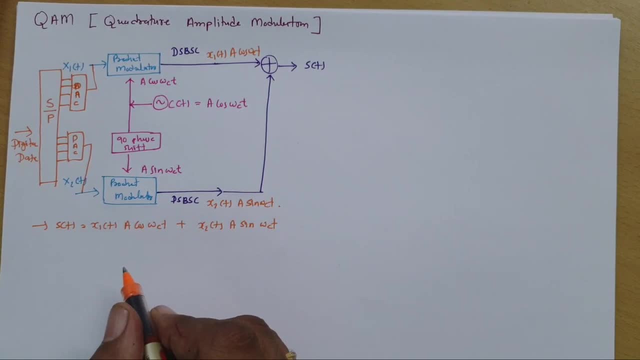 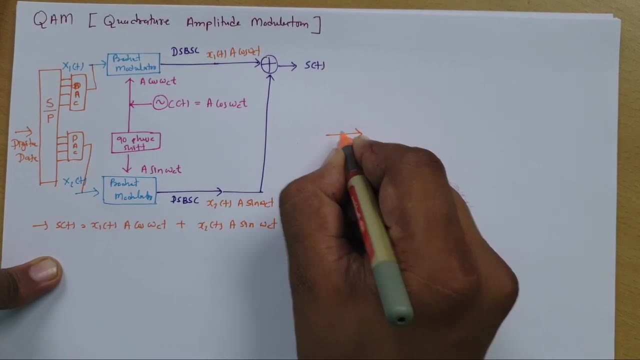 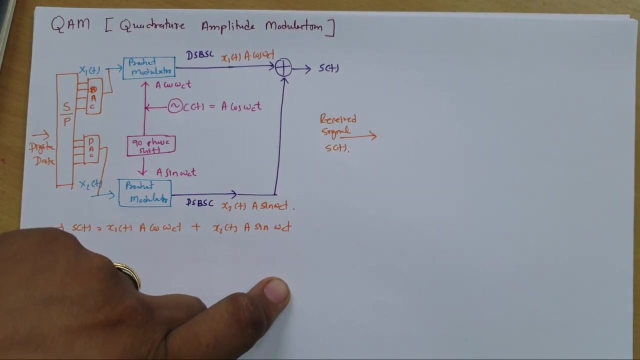 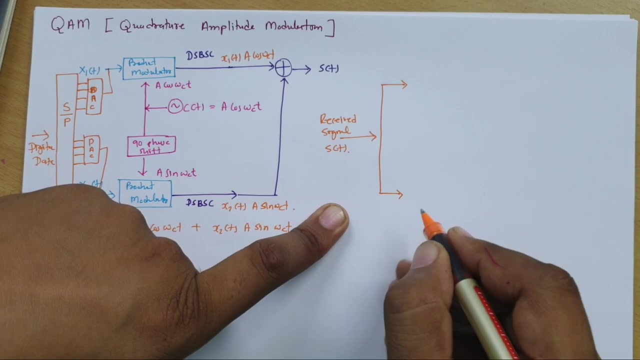 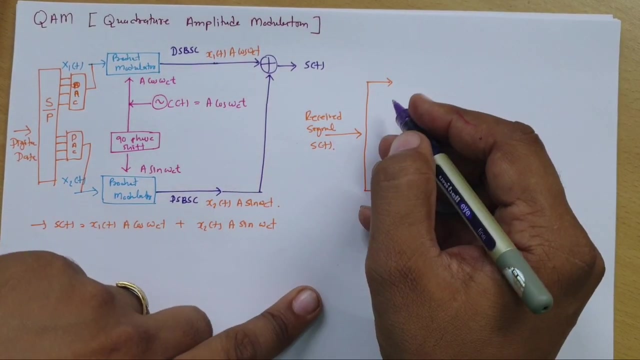 signal that is s of t now let us see what will happen at receiver side. so here we have received signal s of t. right, let us say that is s of t now. this received signal. that is what we will again give it to product modulator and product modulator. second input, that will be carrier signal, which is again 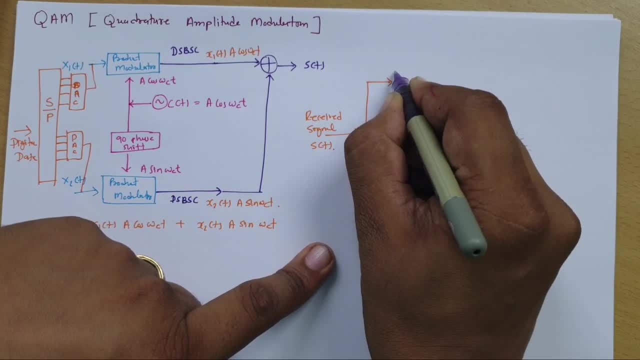 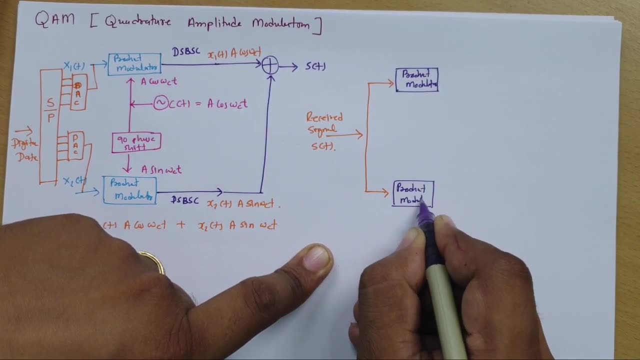 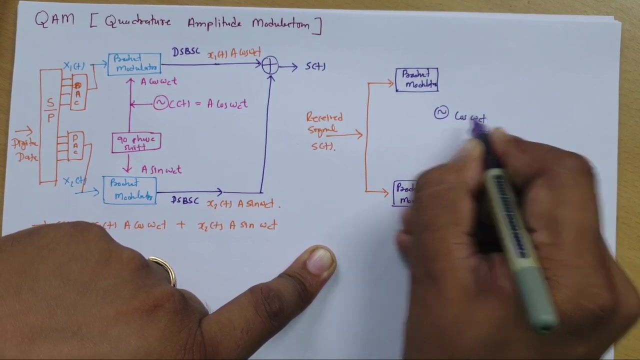 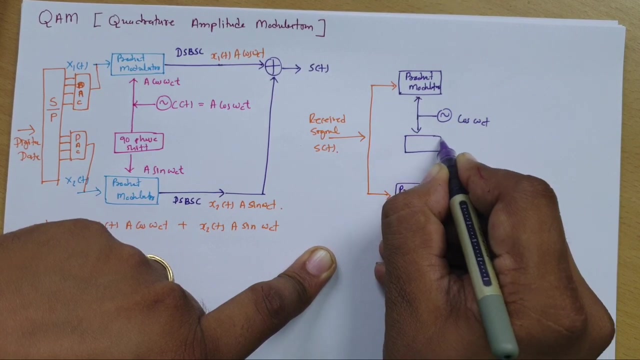 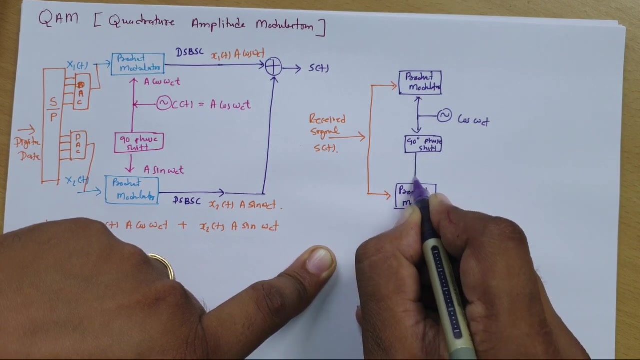 in which is again quadrature in phase right. so here we have one product modulator, here we have second product modulator. let us say we have a carrier signal generator over here, cos, omega ct. one is directly giving it over here and second is given after 90 degree phase shift. so this will be sine omega ct and over here. 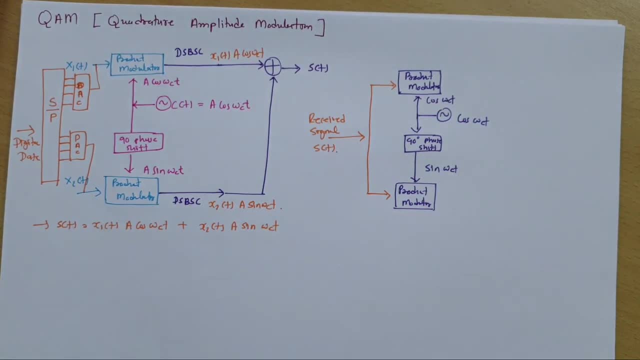 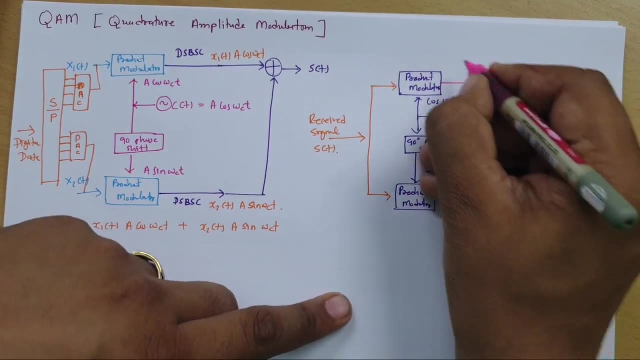 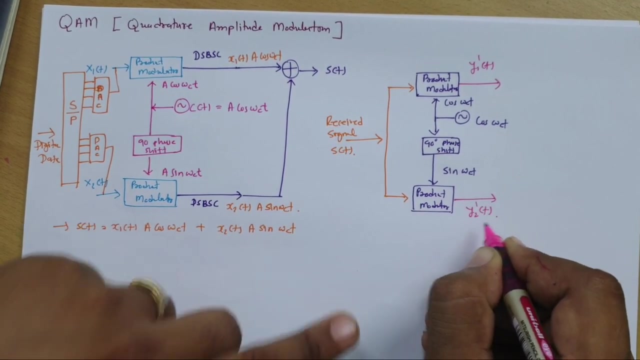 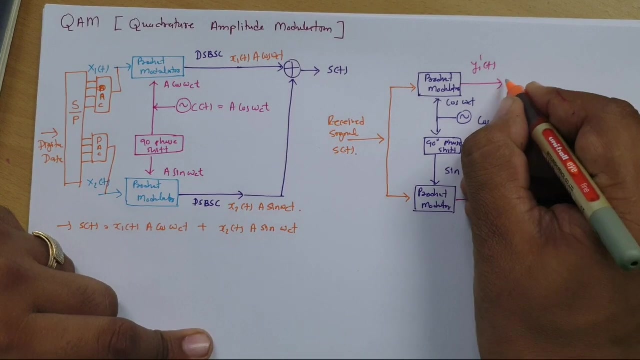 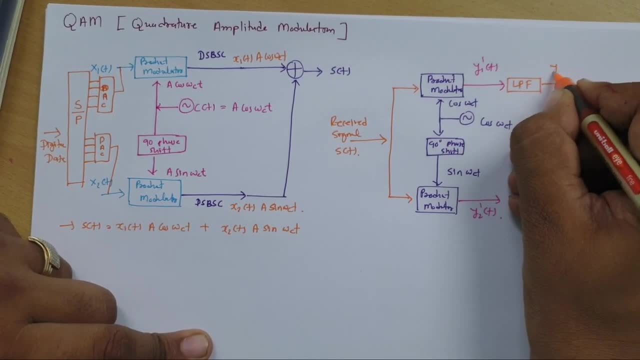 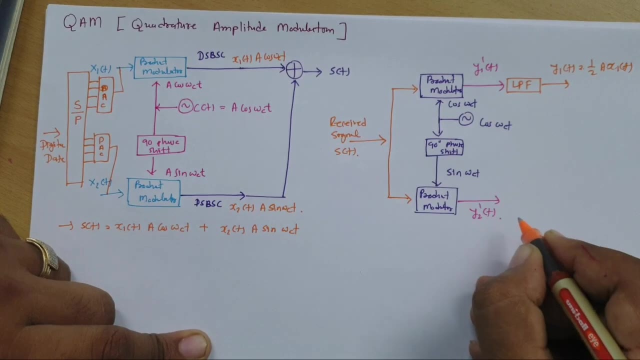 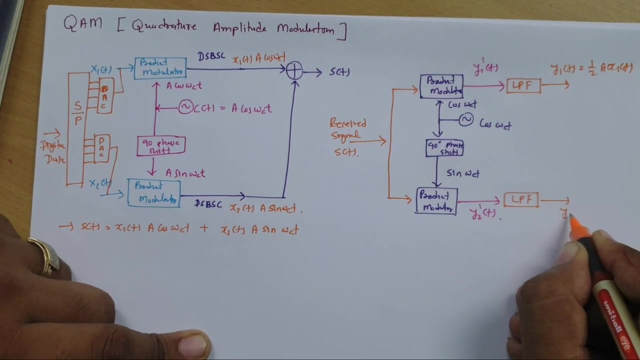 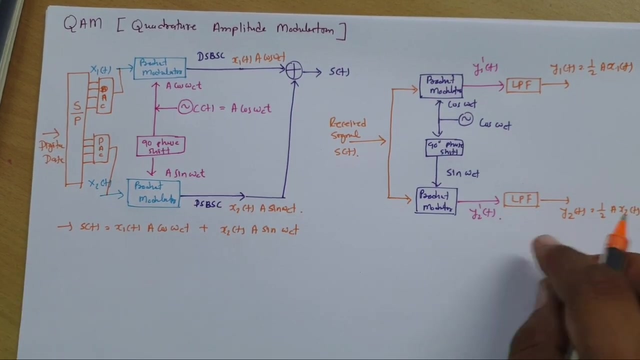 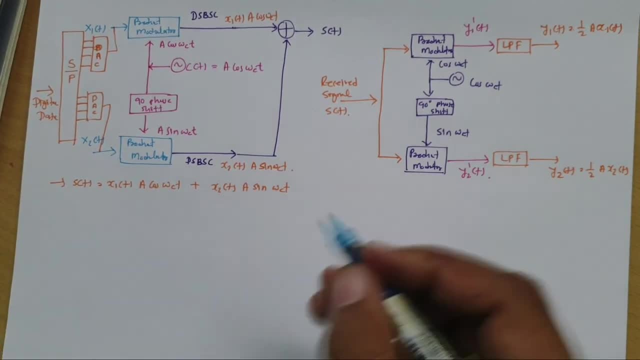 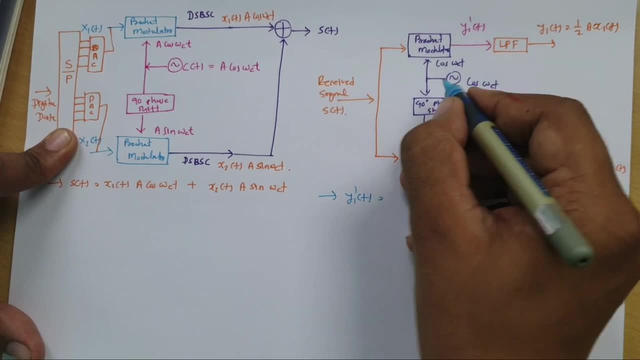 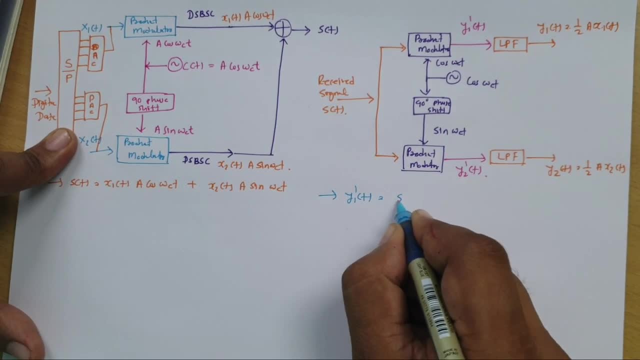 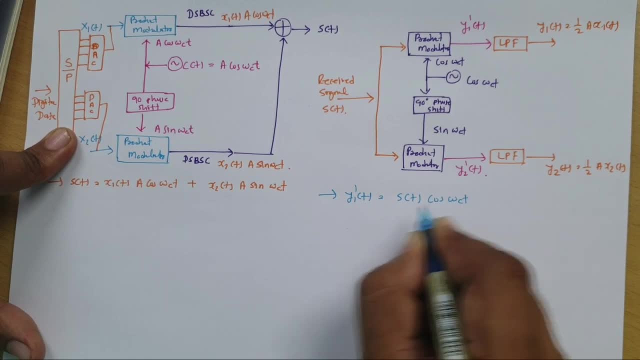